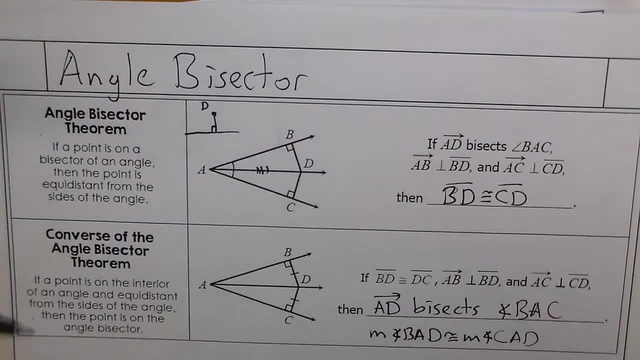 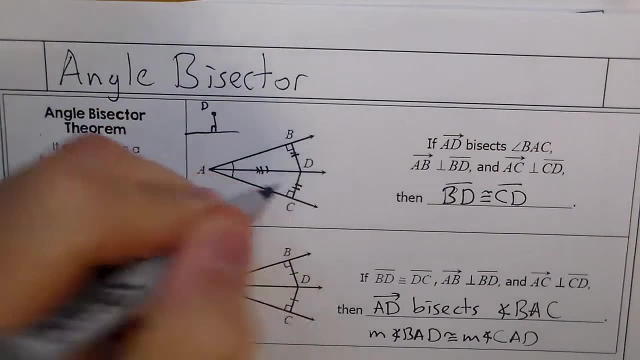 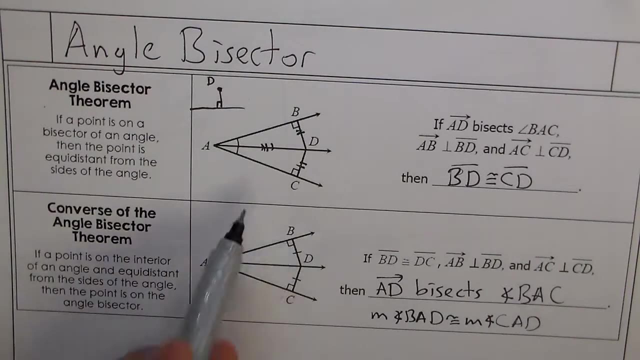 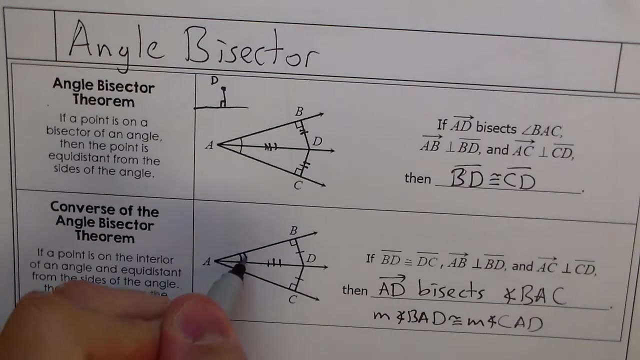 So the background of it is in triangle congruence. Now, in the context of what we're looking at, we're saying that that point is equidistant to the sides. Now the converse of it is saying: if you have an angle and you put a point that is equidistant to the sides, so now it looks like a hypotenuse leg type situation, if we have that, then it's guaranteed to bisect the angle. 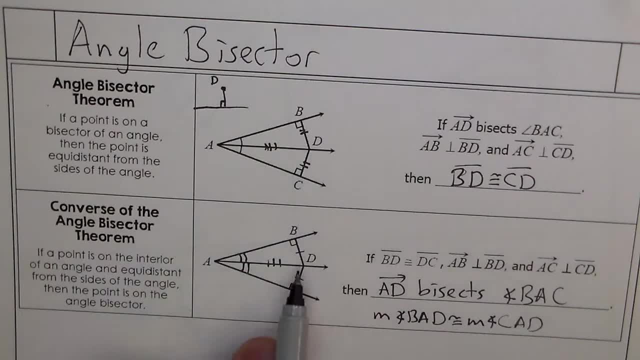 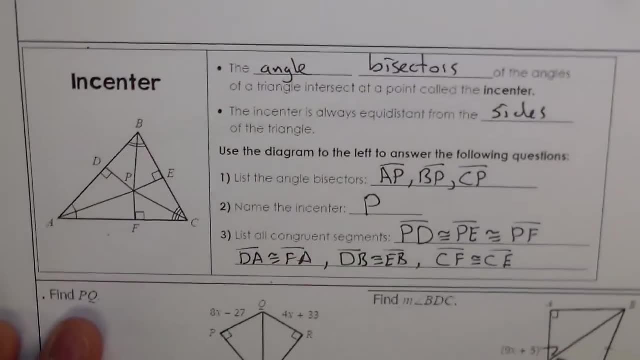 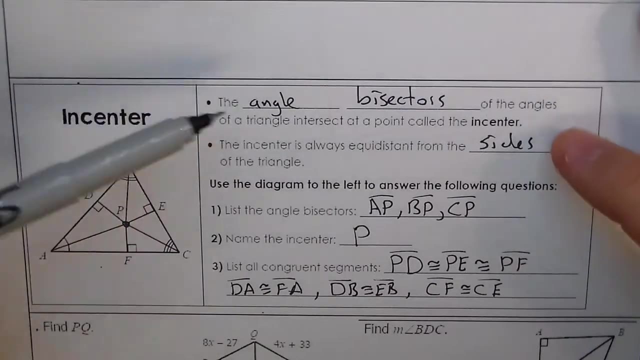 So we start instead of with bisecting: Equivalent we have or equidistant we have. equidistant to bisecting Still works, the same still uses our triangle congruence. Now, when we then take three angle bisectors and put them within a triangle, they all meet at a common point. 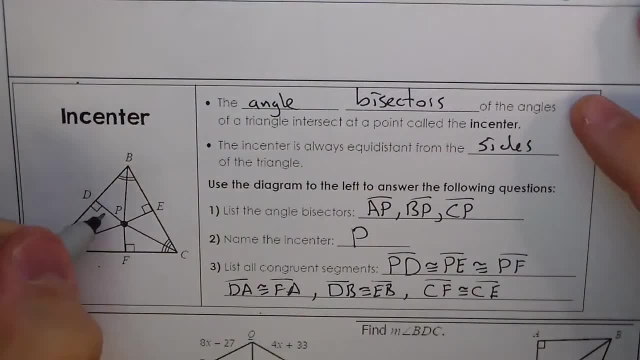 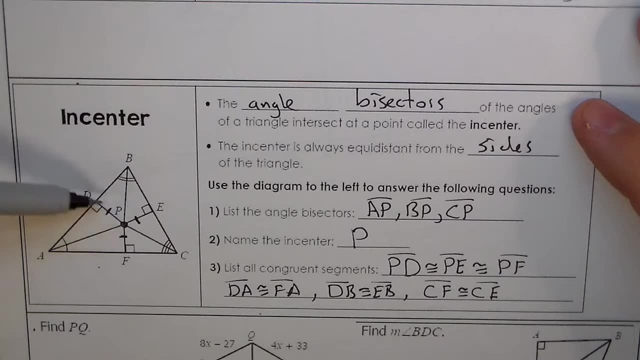 That common point we call the in-center, and you find out that that is equidistant to the sides of the triangle. So where the angles are bisected it's equidistant to the sides. Now I'm going to draw this poorly here. 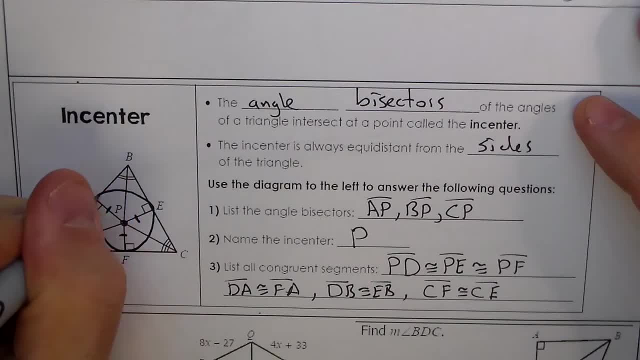 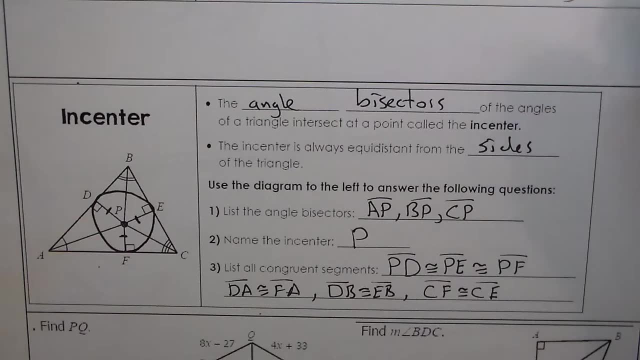 But if I, If I then came in and drew a circle, this point here would be how you inscribe a circle within a triangle, because that equidistant to the sides would be the radii around the circle. Now, angle bisectors are AP, BP, CP. 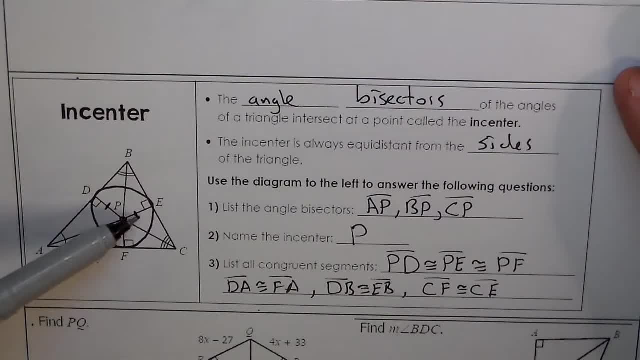 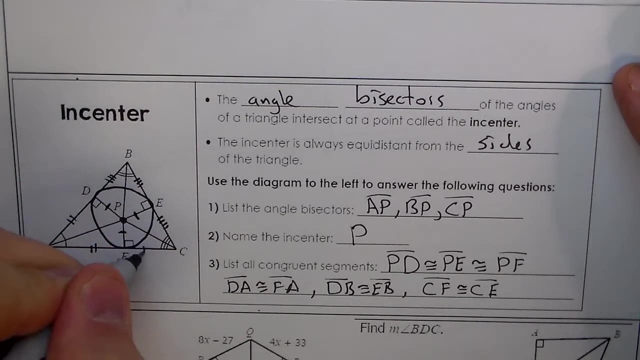 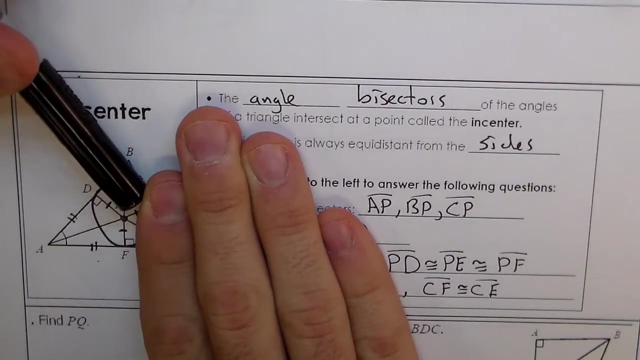 They meet at point P, our in-center, And then I have that equidistant to the sides. but I also have that DA and FA are congruent, DB and BE are congruent And CF and CE are congruent, And that's because this is really almost looks like if we cover up some parts here, this is little kites that I have making them up. 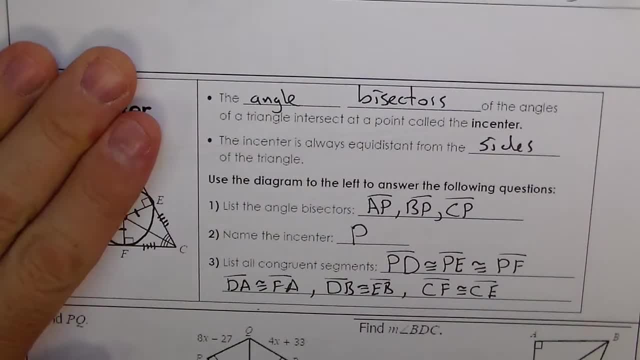 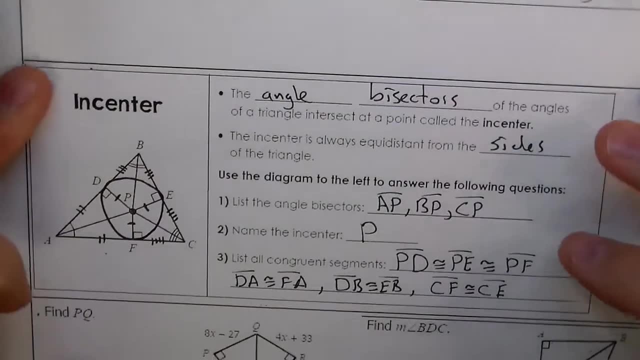 So I have one kite here, There's another kite And then a third one, And that type of congruence works for us as we're looking at the in-center and angle bisectors. Now we'll kind of come back to that. 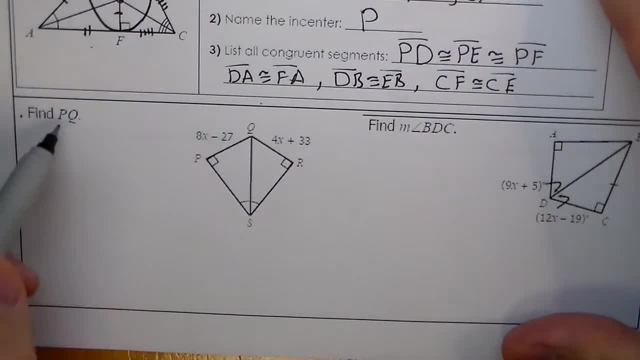 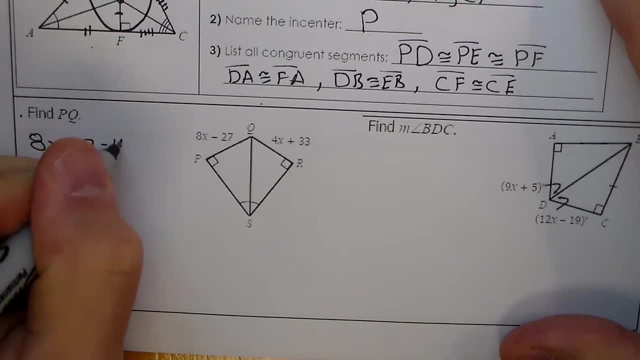 Let's look at just all the angle bisectors by themselves. So I have to find PQ. So this is an angle bisector. We're saying it's equidistant. So we go: 8x minus 27 equals 4x plus 33.. 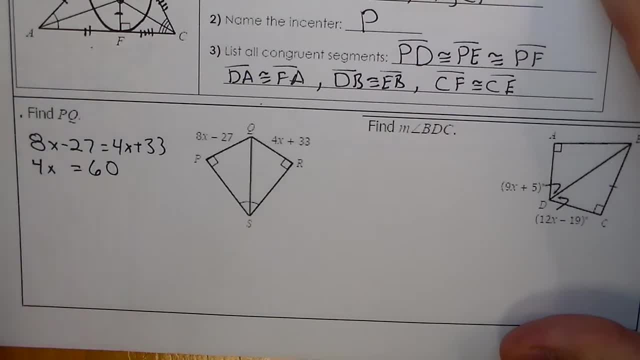 We subtract 4x from both sides and we add 27.. I get 4x equals 60, which gives me x is 15.. So then PQ is 8 times 15 minus 27,, which is 120 minus 27,, or 93. 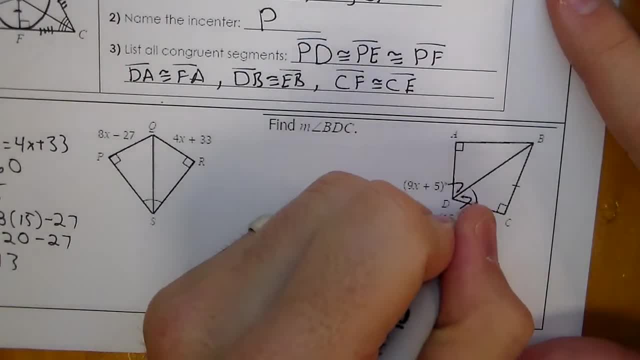 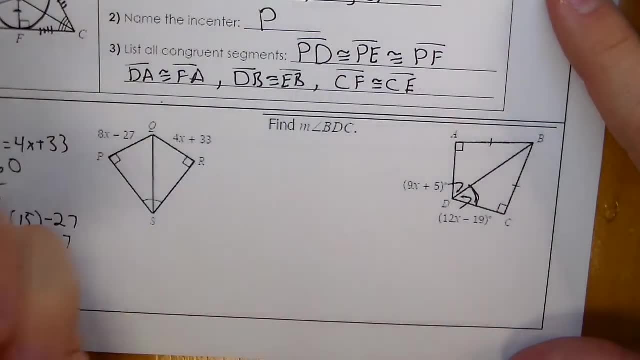 For the next one, the measure of angle BDC, which is this one: right here we're saying that they're equivalent in distance from B to A and B to C, So therefore we can set the angle values equal 9x plus 5 equals 12x minus 19.. 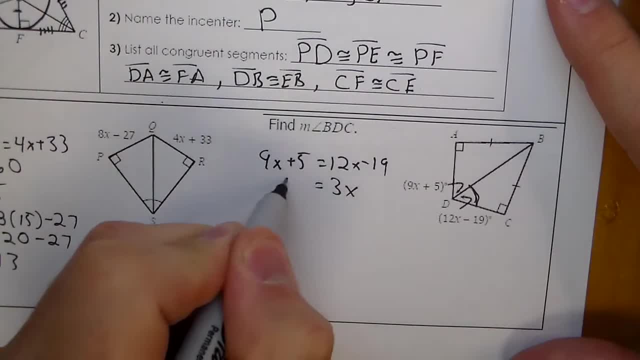 I'm going to subtract 9x and add 19.. We eventually get you x equals 8.. We then substitute into the measure of angle BDC 12 times 8 minus 19.. That gives us 92.. That gives us 96 minus 19,, which is 77 degrees. 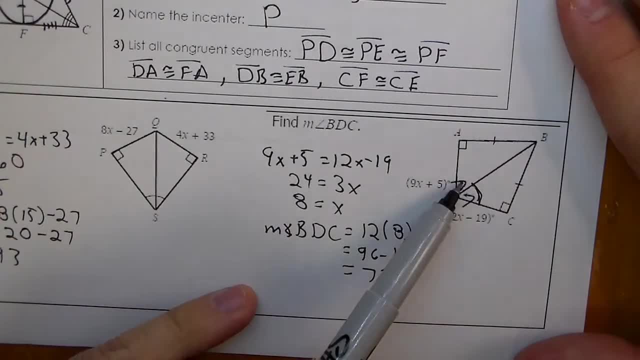 Now you may be asked to find other angles here. If this is 77, this would also be 77.. Together, 154.. Since I have a right triangle and this is 77, that's 13 degrees because I have to add to 180. 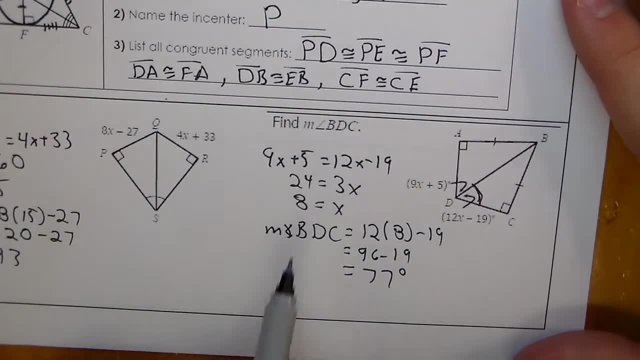 That would be 13 degrees and then 26.. So just be careful. what it's asking for, Finding x- is very good, but you've got to make sure you answer the question that you're given. For our next one, we need to find x. 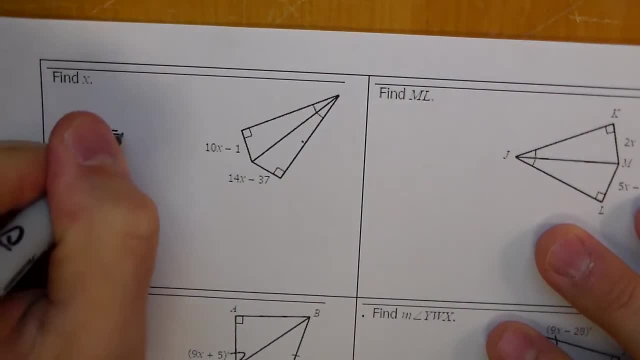 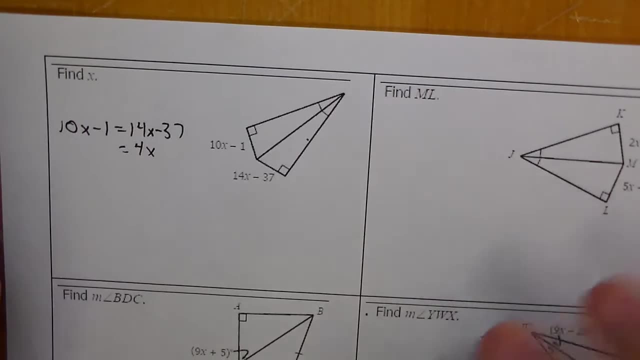 They are corresponding congruent parts. 10x minus 1 equals 14x minus 37. I'm going to subtract 10x. I'm going to add 37 to both sides, I get 36.. So that gives me x equals 9.. 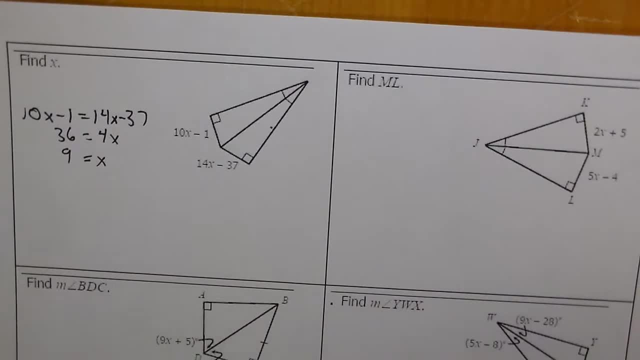 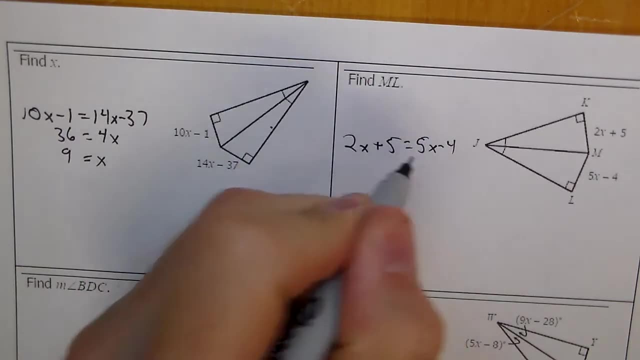 I didn't need to substitute in, That's all I needed. Next one I need to solve for ML. I'm going to say 2x plus 5 equals 5x minus 4.. I'm going to subtract 2x from both sides. 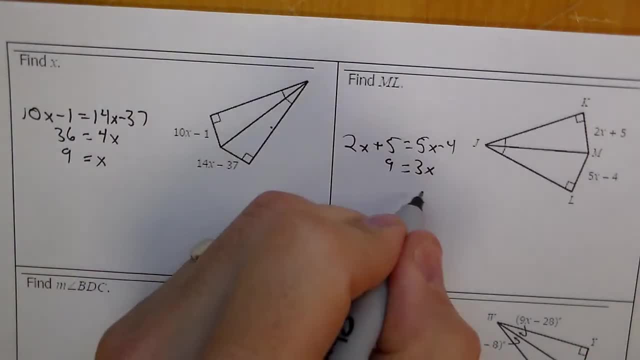 We get 3x, I'm going to add the 4.. I get 9.. So x equals 3.. Now ML, we're going to substitute into 5x minus 4. So that's 5 times 3 minus 4.. 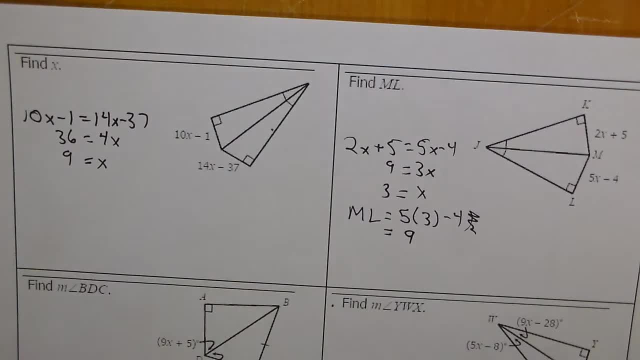 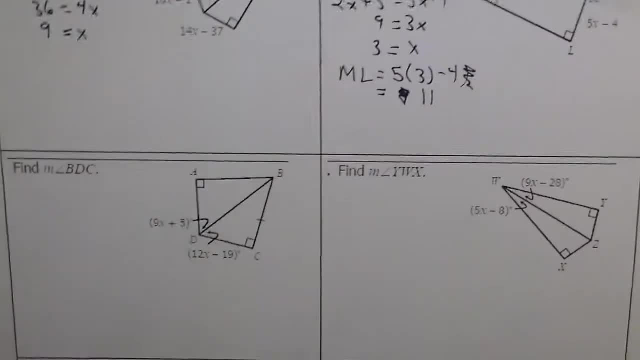 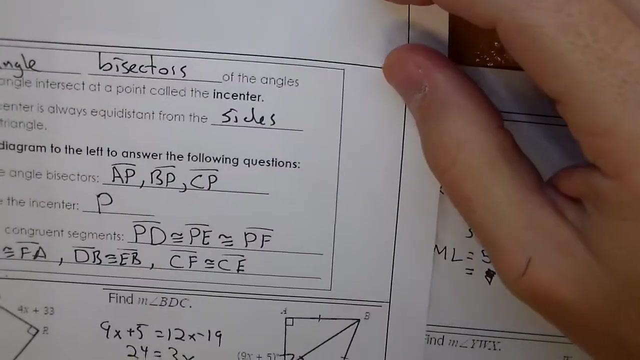 15 minus 4 gives us 9.. No, it doesn't, It gives us 11.. For the next one, this was the same as the previous problem. If you've noticed that it's right there, It's 77.. 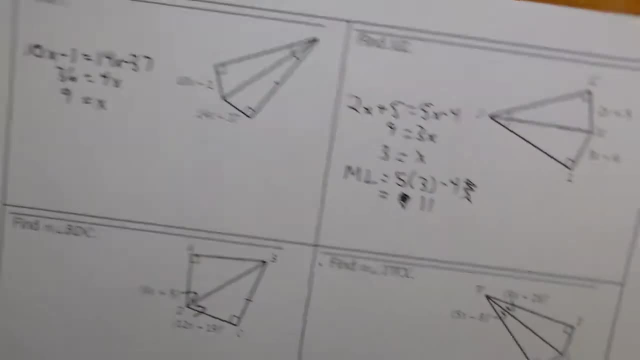 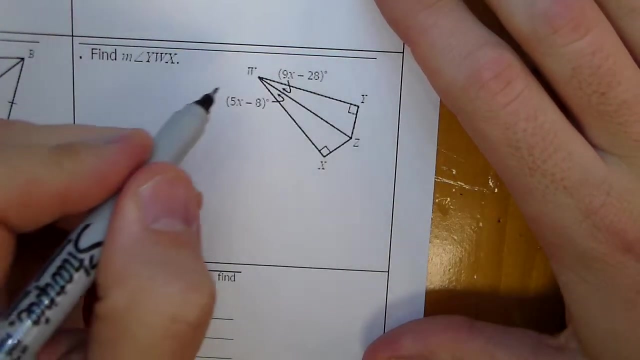 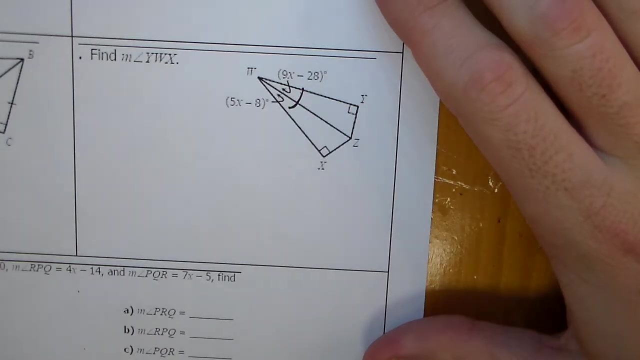 We don't need to solve that one again. It's the same as that bottom one on the first page. Let's go here: The measure of angle, ywx, which is the whole thing. So I'm going to have to find each angle and then substitute in after I find x and find the total. 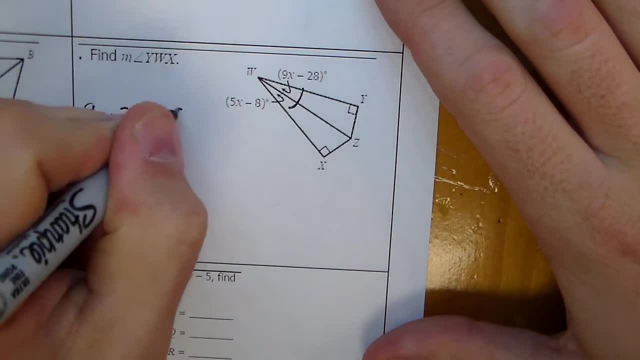 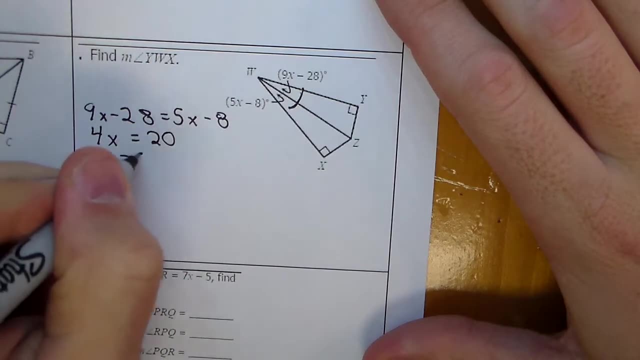 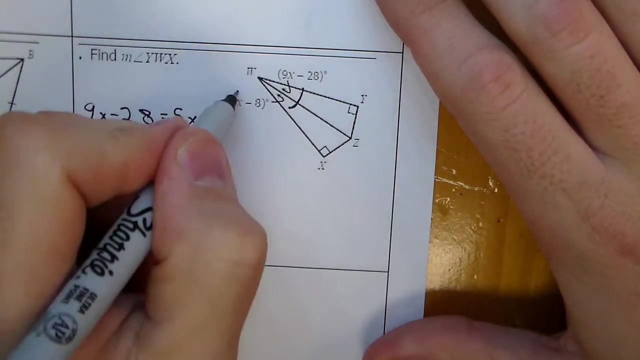 So we're going to go: 9x minus 28 equals 5x minus 8.. We subtract 5x, We add 28.. We get x equals 5.. Now, when we substitute that in, I get 25 minus 8, which is 17.. 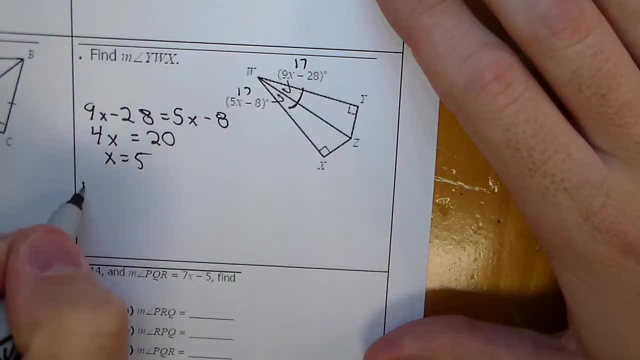 Then I get 45 minus 28,, which is also 17.. So the measure of angle ywx would be: you could combine the two and make it 34 degrees. Last part: here I have to find a bunch of angles and I start with some values here. 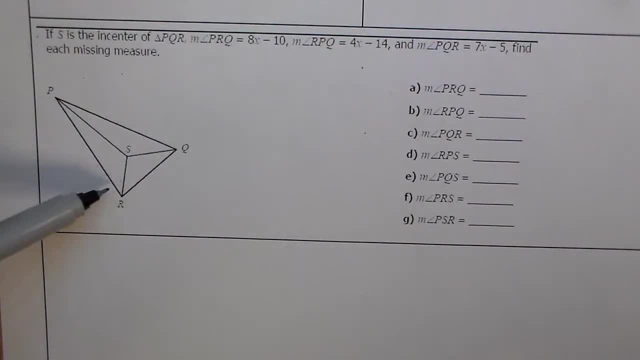 So PRQ, which is the angle at r, RPQ, the angle at p, And PQR all have expressions with x in them. Now I know these all add to 180.. So I'm going to start with that: 4x minus 14.. 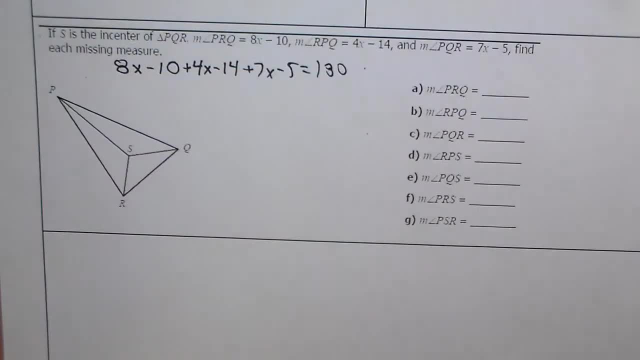 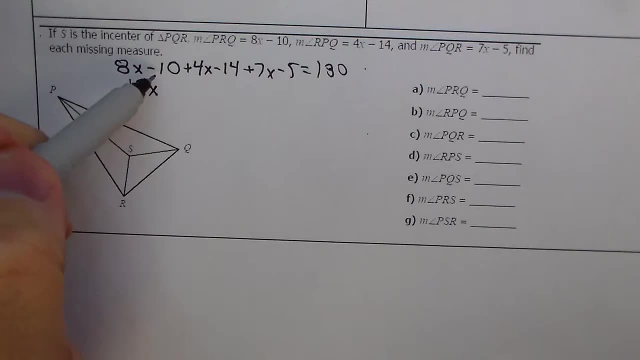 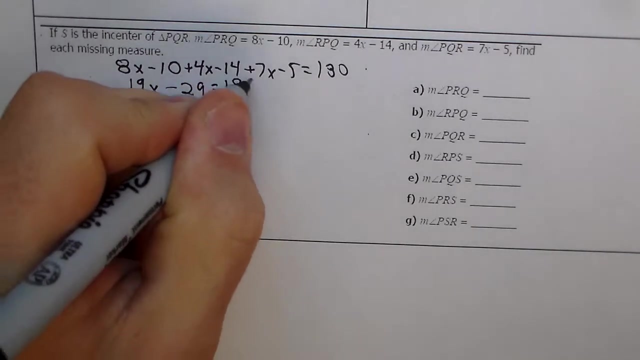 7x minus 5 equals 180.. So we have 19x. That looks like a Minus 10 minus 14.. That's minus 29 equals 180.. So we're going to go: 19x equals 209.. 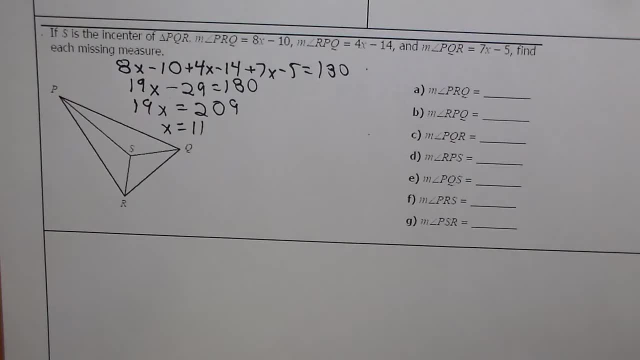 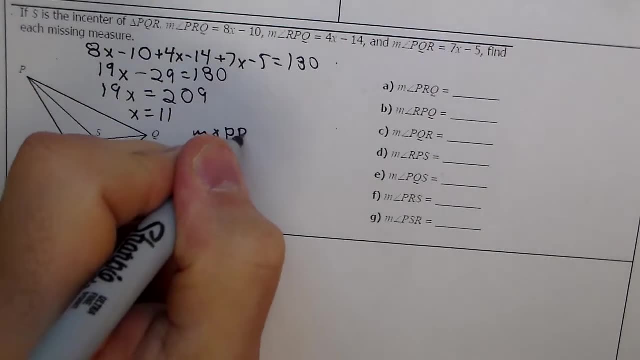 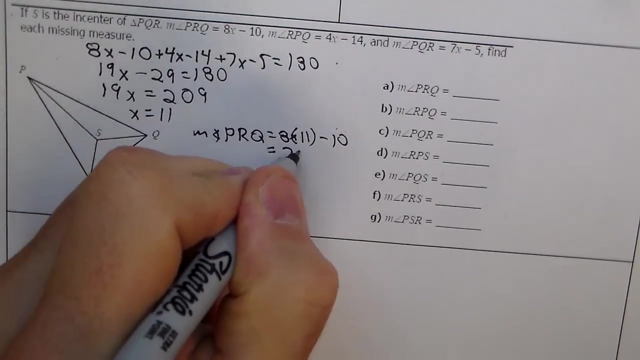 So x is 11.. So if x is 11, I need to go back and find the angles. So the measure of PRQ, or 8x, 8 times 11 minus 10, is going to be 78.. 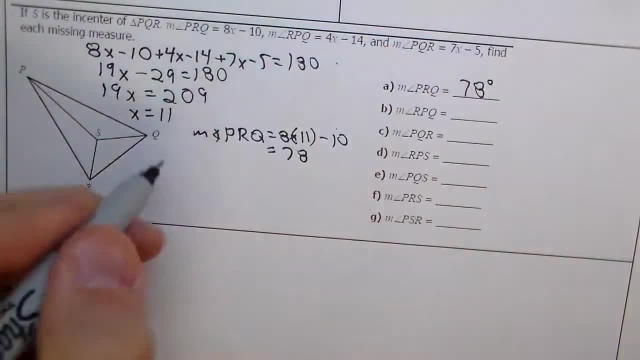 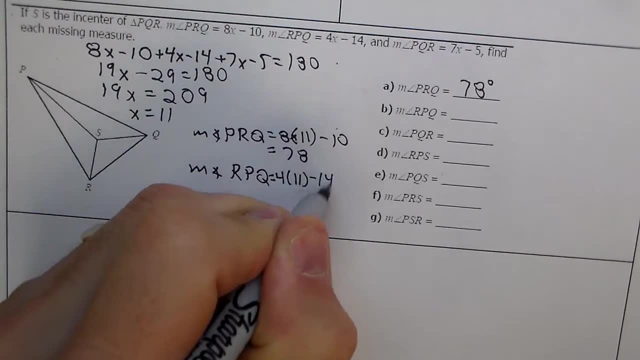 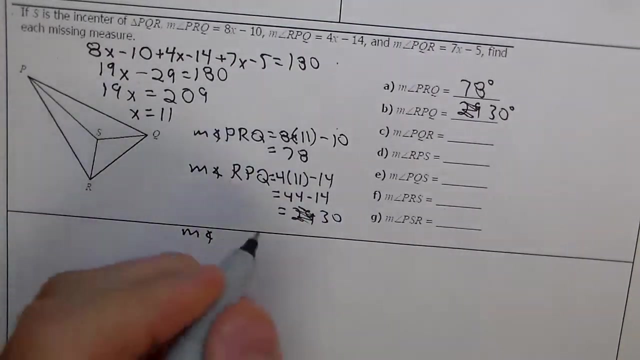 78.. The measure of angle: RPQ 4 times 11 minus 14,, or 44 minus 14,, 29.. And the measure of angle, That's not 29.. Let's try again: 30. And the measure of PQR.